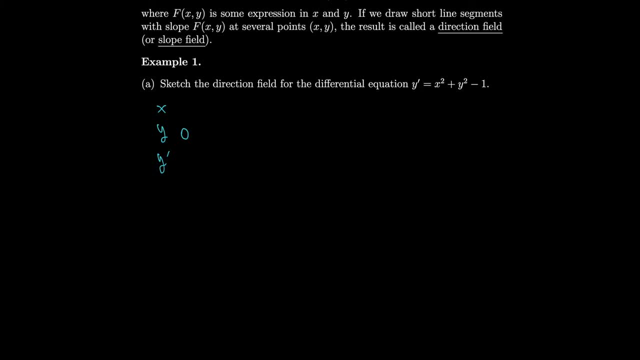 a bunch of y values at zero, We can look along the x-axis first. So when y is zero, and let's look at how about x is minus one and y is minus one, and x is minus one and x is minus one. 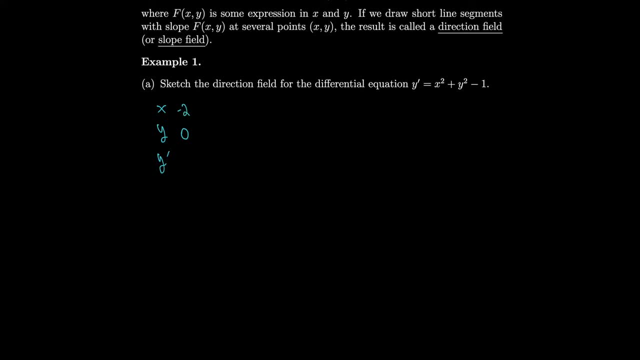 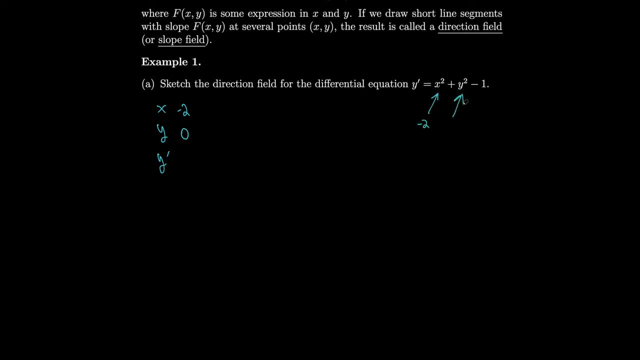 in and we plug in 0 for Y, so we end up with 4 plus 0 minus 1, so Y prime becomes 3, so that means that we should draw some axes and a little lower and go for the back a little bit. we've got going up to here's one. there's two minus one and 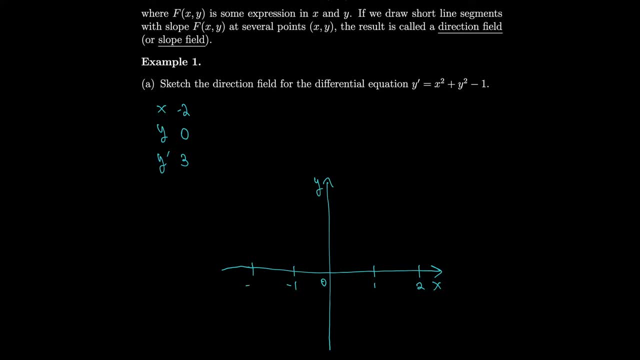 minus two mm-hmm. they'll make this a little bit farther. okay, so we just did minus 2: 0. so that means that there's a little line segment at minus 2 that has a slope of 3. so instead of drawing an entire line with slope of 3, which would look like I. 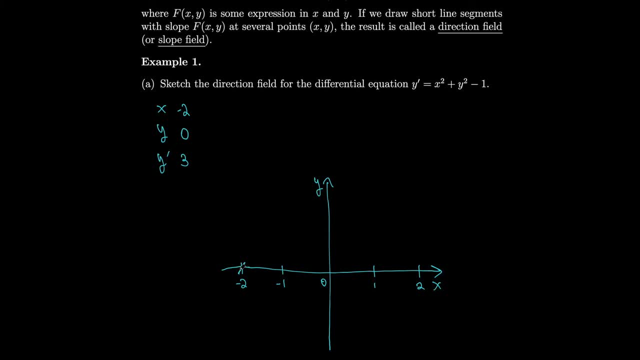 don't know something like that. so draw a tiny little line segment with a slope of 3, and then I do my next point. I'll go to still along the x-axis, so I'll still go along. y equals 0. I'll go to minus 1. 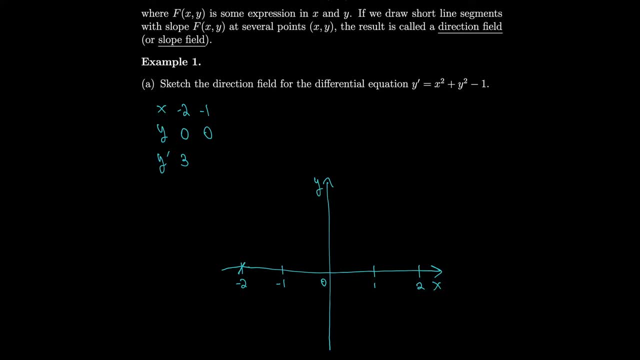 now, well, plugging in minus 1, I squared that plus 0 minus 1, so the slope is 0 over there. so I should make a nice segment over here with slope 0 at minus 1, so nice horizontal little line segment, and then at 0. I can see that I'm gonna. 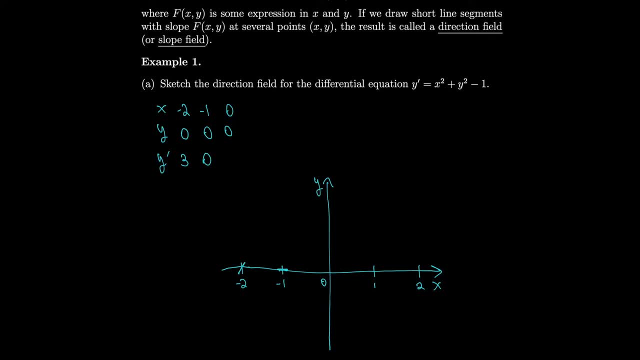 go for 0 for Y, also because I'm just choosing any two points for these guys, because there's no otherocks to nests, they're just for this one. so I will go back over to minus 1. so this is just smarts, so I don't have anything to pull. 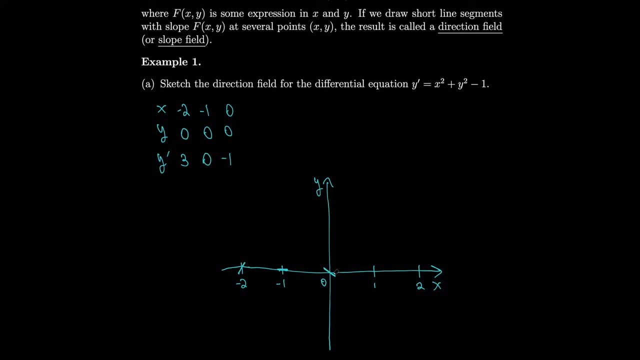 over here to my advantage. so if I'm readings 4, if I go over here to minus 1, right at that point I won't have any coaster. so at this point you can draw the whole thing. but this just is a quota and I can still go in and select this loss. 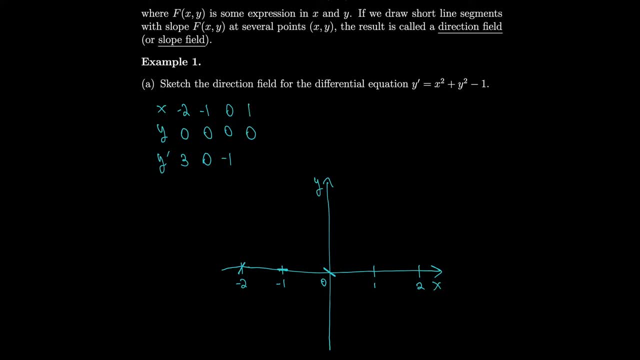 which can only be done if you go to minus 1. that is the last step where you would be able to Draw to our usual line segment畫อ, number 1. this Indice 2 equals 1, X, 2 Insurance. 1 is what we'd read, as y is, 1 is usually less than y. 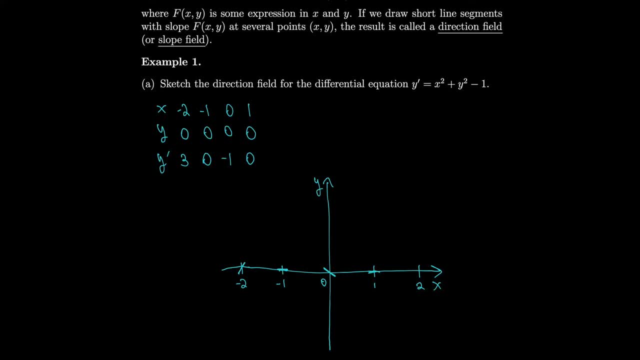 and then at 2 we should get. if we plug in 2 and 0, we get 2 plus 1 is 3. sorry, 2 squared is 4 minus 1 is 3. so I should get another line segment of 3 over there. 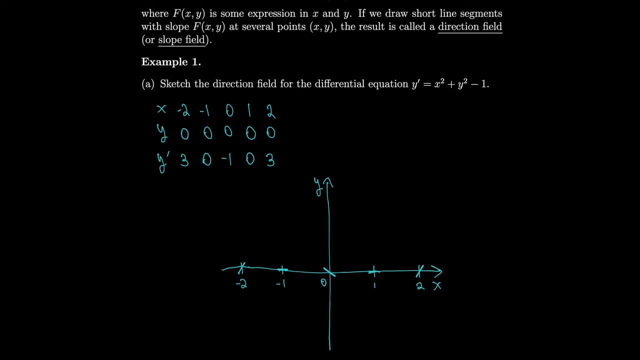 and you keep doing this, so we get. if we want the next row, we could do minus 2, 1 this time instead of minus 2, 0. you plug that and you get 4 for the derivative, so the slope is 4. 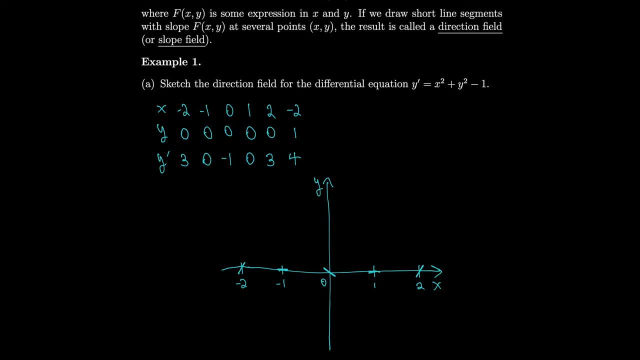 so minus 2,, 1, I should make this. let's see if I can make this even steeper. actually let me go higher. so if this is 1, so I'll make this over there pretty steep, because it's a slope of 4 now. 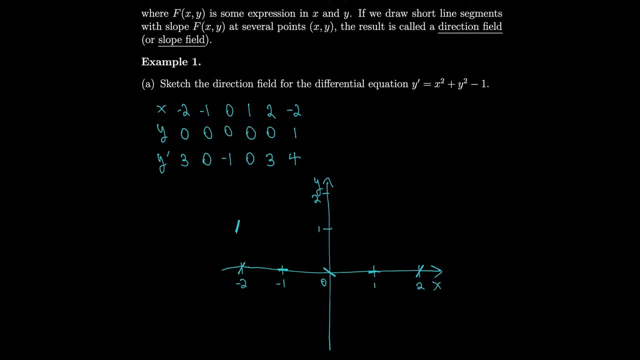 and let's say there's 2, so you can keep going like this and fill in the rest of the table and the rest of the slope field. you don't have to limit yourself to the table. once you get used to it you can just start making all of these. 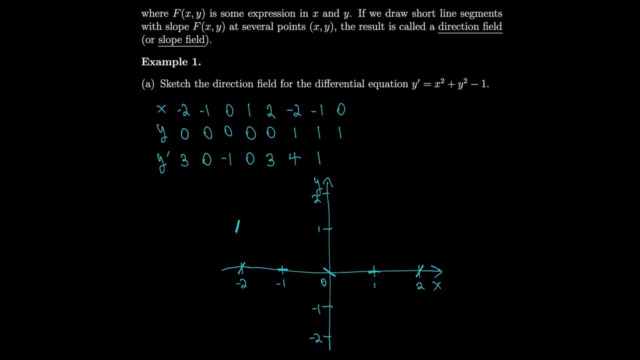 slopes in your head. you can compute all of the derivatives in your head without having to actually write down the table, but it's, I think, nice to see how it works out and see it all in action. so you should end up with something roughly like that. 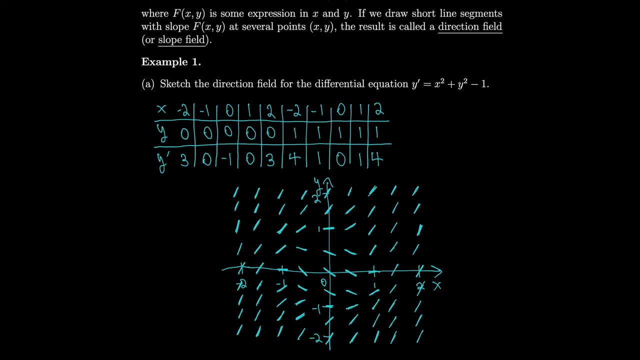 notice that after I finished with you know integer points from minus 2, minus 1, 0, 1, 2. I went halfway in between, also just to have a more complete graph and you can see why I only went up to 2. 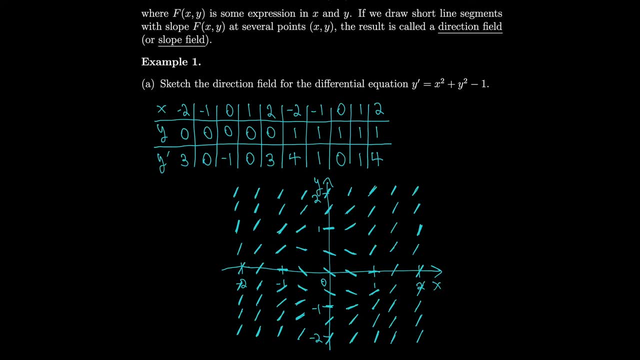 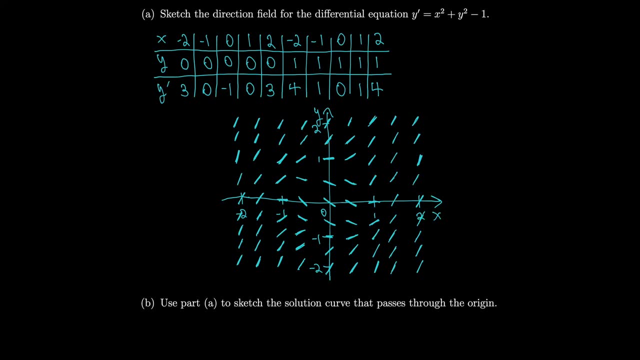 because this is very labor intensive to make one of these things by hand. let's do the second part of this problem now. we'll use part A to sketch the solution curve that passes through the origin. so, as you've seen before, for a differential equation there are lots of little potential solution curves. 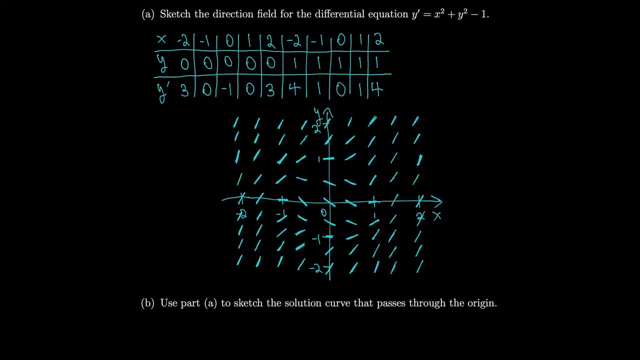 you could start almost anywhere you want and then go through it. all depends on your initial value, usually. so we want the one that passes through the origin. so we want the one that passes through the origin. so let's look at the origin and let's follow along. 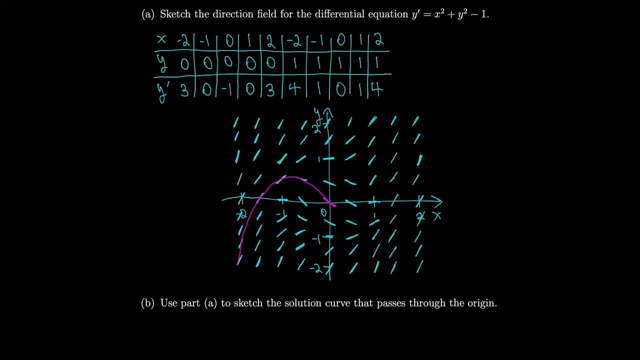 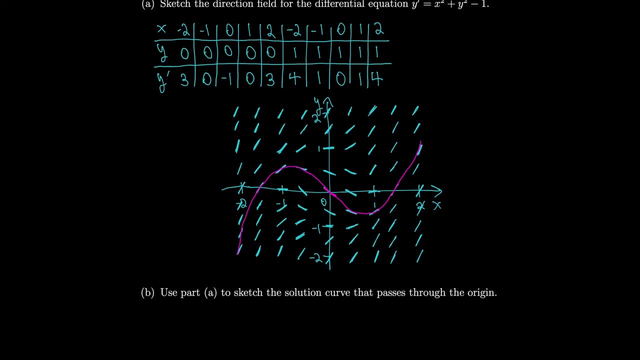 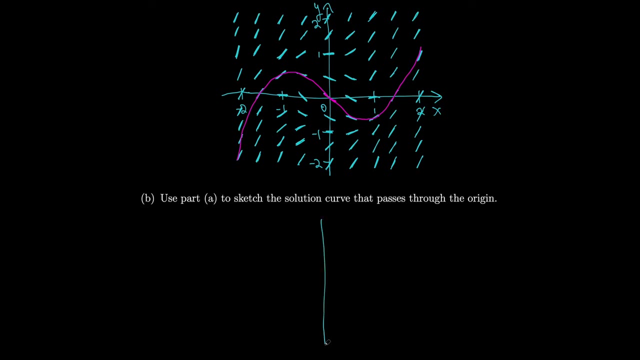 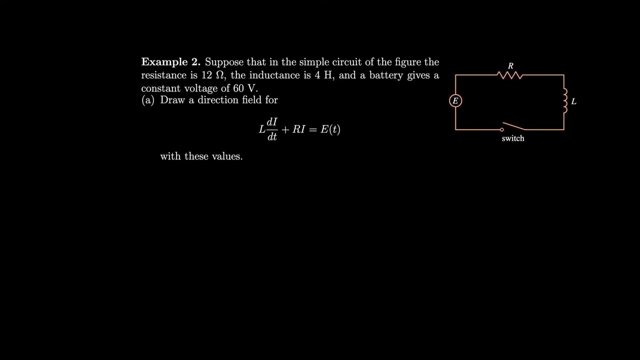 the path. so we do that and we roughly get a solution curve like that. so I think that we can draw that. now it looks like our solution curve should be this polynomial-like looking thing, or it could even be a trig function. suppose that in the simple circuit of the figure. 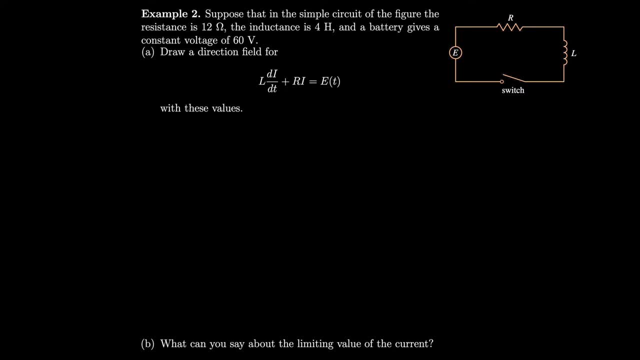 the resistance is 12 ohms, the inductance is 4 henries and a battery gives a constant voltage of 60 volts. let's draw a direction field for L times. di dt plus Ri equals E with these values, so that means that L is 4. 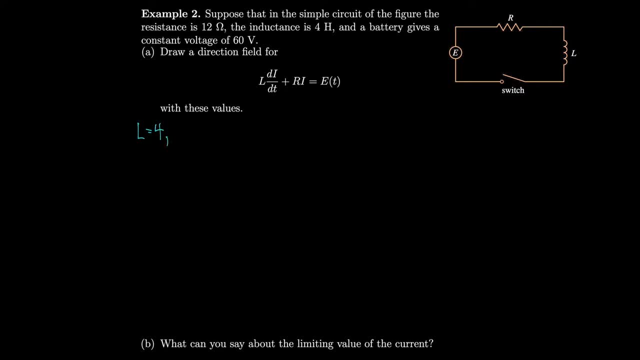 because our inductance is 4 henries. we have that our resistance is 12 ohms, so R equals 12. and we have that our voltage is a constant 60 volts, so E is a constant 60. so if we plug that in, we get. 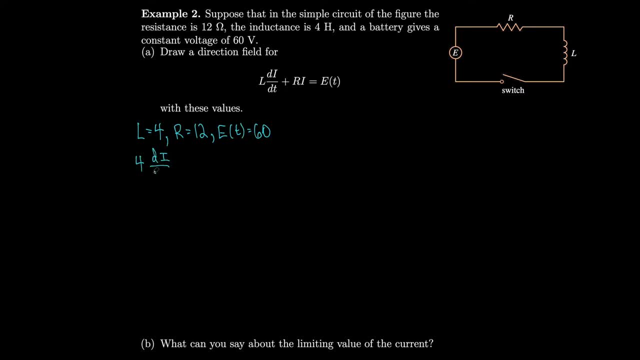 4 times di dt plus 12i equals 60. in this case, i is our y and di dt is our y prime. so di dt is equal to 15 minus 3i. so if we draw a slope field it should look roughly like this: 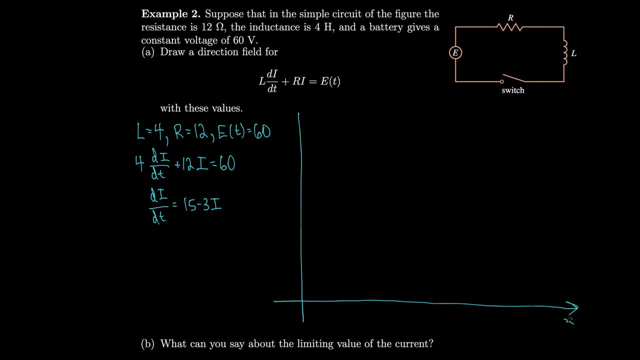 very roughly. that's not t, though, sorry, it's not x, it's t, and this is not y, it's i. so if we look at 15 minus 3i, you can see right off the bat by inspection: if i is equal to 5, then the slope is just 0 all the way through. 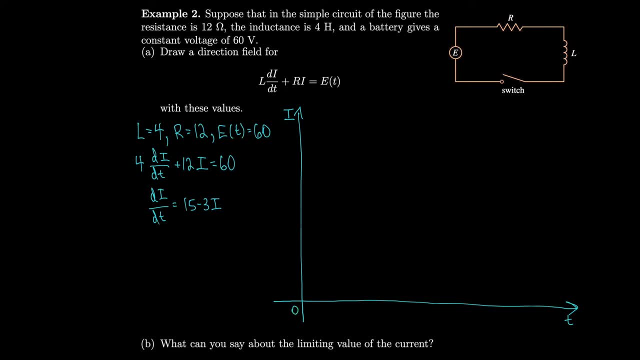 so how about I start with that? I'll go 0, I'll go 1, 2 and 3, and I'll go 2, 4 and 6. how about? so? constant 5? sorry at i equals 5, it's a constant 0. 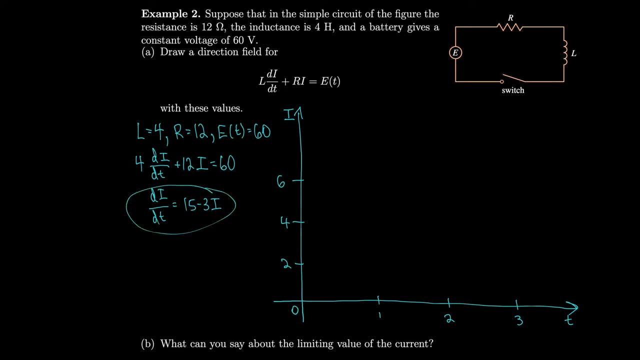 for the slope, because plugging in 5 gives di dt equals 0. so I'll just draw a whole bunch of little line segments with slope 0 and then if I go a little bit higher- let's say I went to 6, 15 minus 3 times 6- 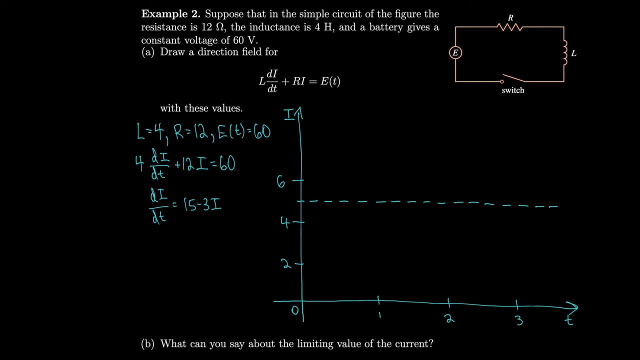 is negative, because 15 minus 18 is negative 3, so this is a slope that's going down 3, and it doesn't matter what the value of t is, because e of t was constant 60. so no matter where I go, this thing will be. 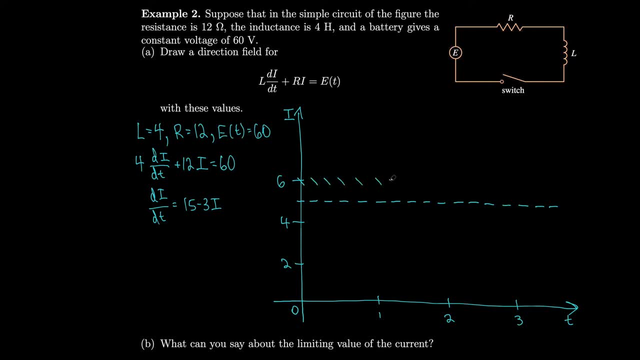 constant slope of negative 3. so I'll just draw all of those little slopes. if I look at, let's say, 4, 15 minus 3 times 4 is 15 minus 12 is positive 3. so I can just draw the reverse and then I can fill in the. 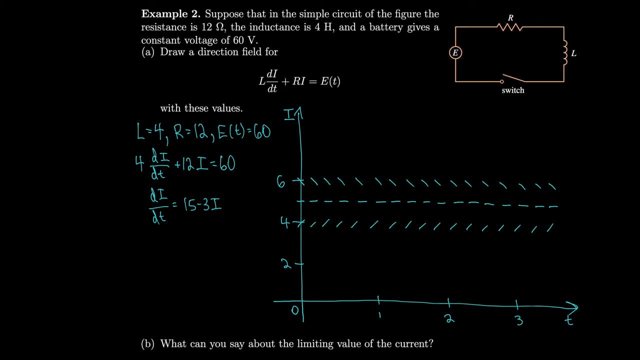 rest of the slope field similarly with this one, by just looking at different i values, because it doesn't matter what t value is. all of those slopes along with that same i value are going to be parallel, so you should end up roughly with a slope field that looks like that. 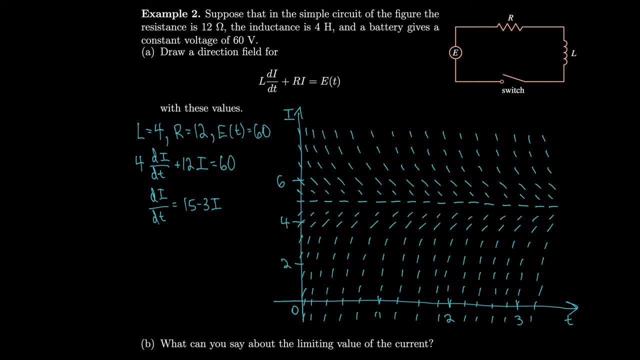 let's see what we could say about the limiting value of the current. it looks like any slope field we draw, so we drew one like this or like this, or one like this or one like that. they would all end up stuck over here, not going past 5. 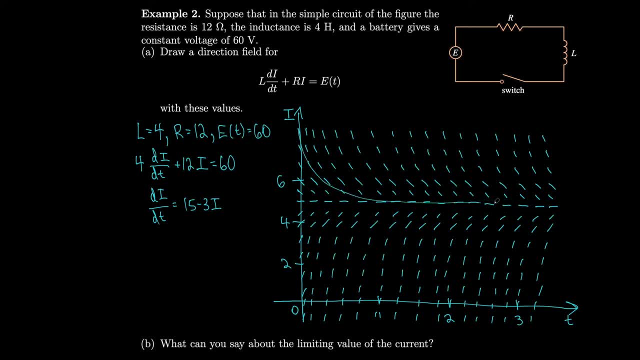 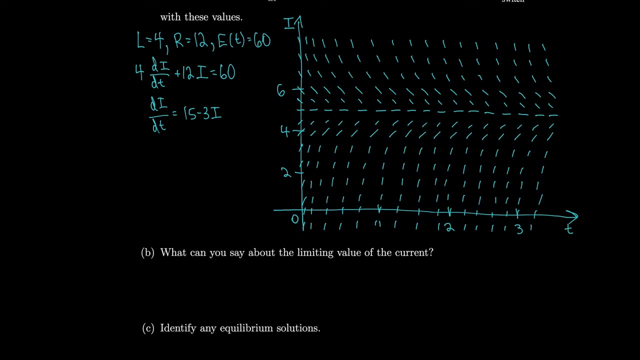 similarly, if we drew slope fields coming out over here, they would still not go past 5. they all just kind of end up corralled at this limiting value of 5. so it looks like all the solution curves approach 5 amps, so we could say the limit. 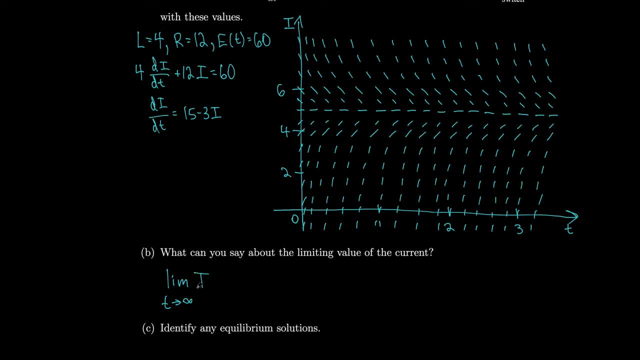 as t goes to infinity. of any solution, curve i of t should equal 5. let's identify any equilibrium solutions. equilibrium solutions are solutions that make our rate of change stop. once the rate of change is 0, then nothing is happening anymore and everything is at equilibrium. 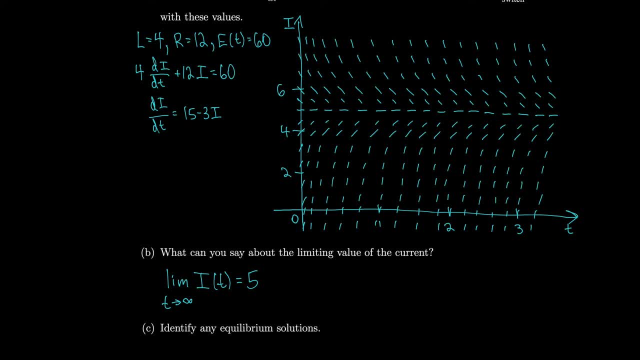 so let's see what makes our di dt equal 0. well, that was how we started drawing this thing in the first place. we noticed that plugging in 5 makes this thing 0 if you look at the solution curve that goes over here, that solution curve. 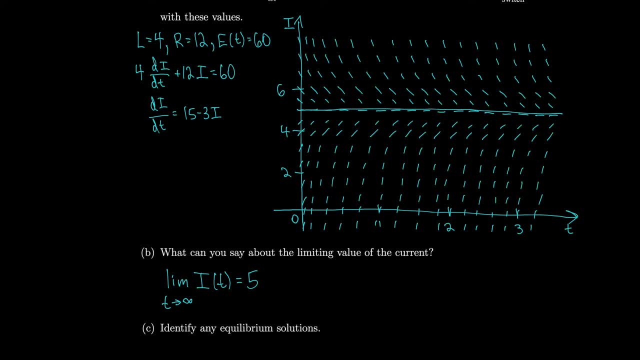 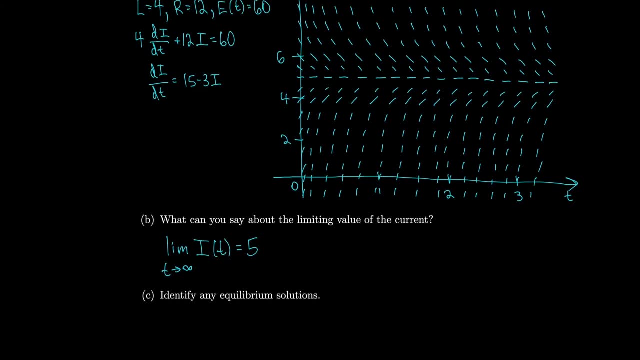 cuts through every single 0 slope line segment. so that's an equilibrium solution. so we can say that when i of t is 5, that implies that di dt would be equal to 15 minus 3 times 5, which is 0. so that's an equilibrium solution. 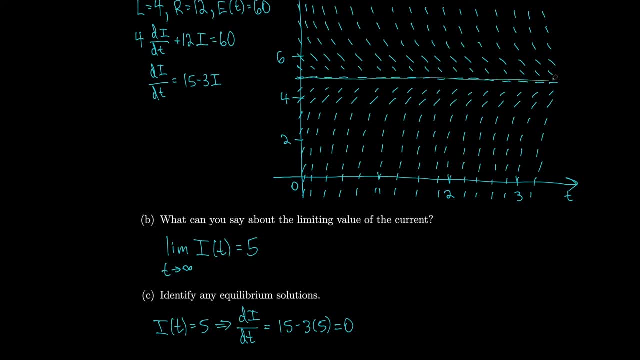 equilibrium solutions don't have to just be straight lines, though, in general. let's say you had a differential equation that actually had some of your independent variable involved. in this case there's no t, there's just i and di dt. but let's say you had something like: 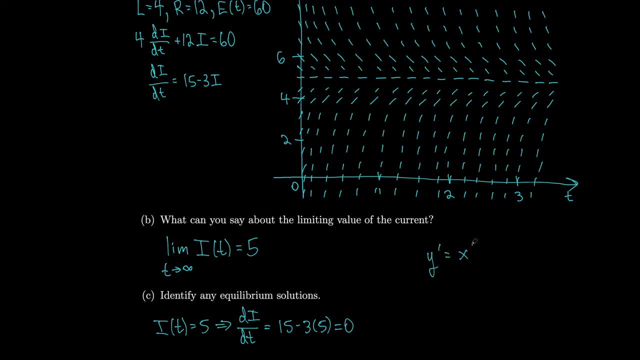 y prime equals x squared minus y, then in that case you would expect an equilibrium solution for y to be x squared, because plugging in x squared would give you 0. x squared minus x squared would just cancel. so in that case you would expect that your slope field 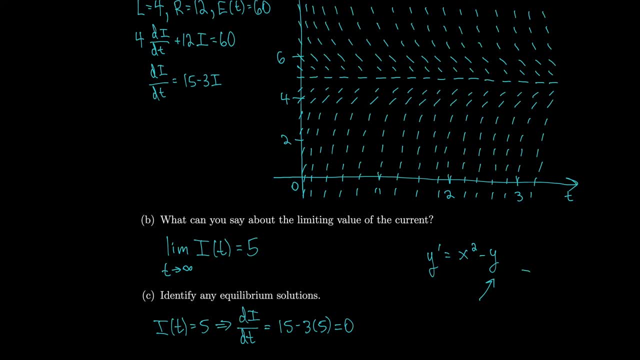 would have a whole bunch of 0 slope line segments in the shape of a parabola if you were to draw them for that particular solution curve. but i digress. our example just happened to be that our equilibrium solution was a nice straight line. if the switch is closed when t equals 0. 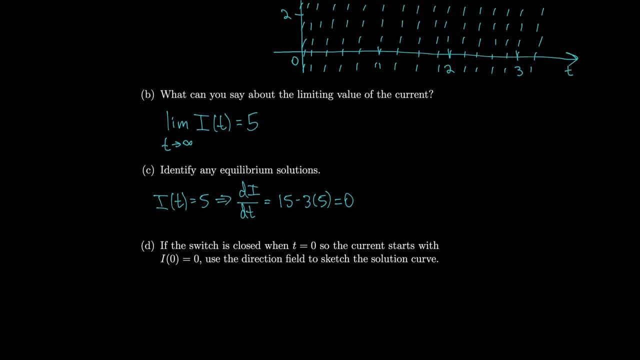 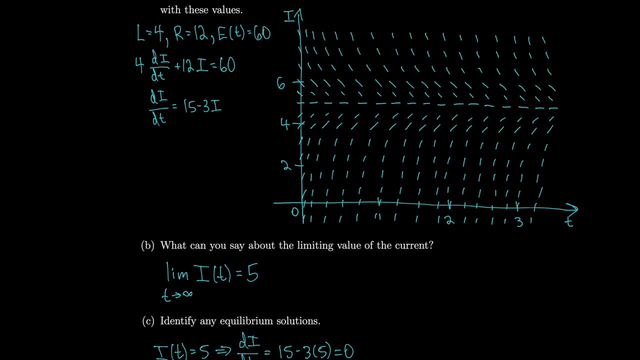 so the current starts with i of 0 equals 0. let's use the direction field to sketch the solution curve. so we go back over here. we're going to try to sketch the solution curve starting at 0. so we're starting at the origin, looks like if we follow the flow. 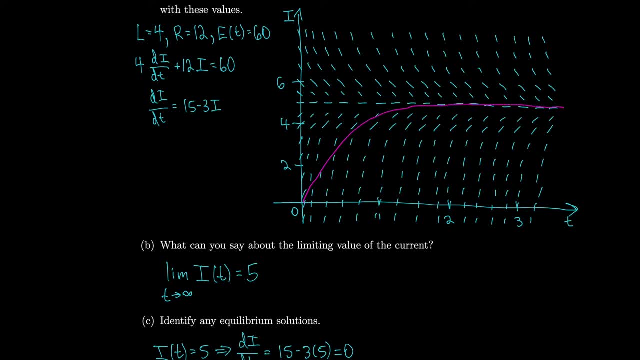 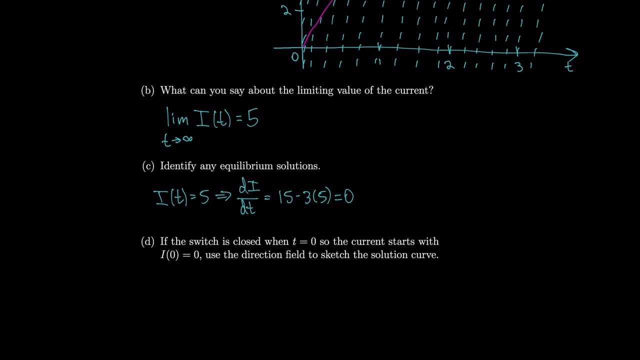 then it looks something like this for our solution curve, so we can bring that down over here. it looks like: if here's i and here's t, then here's our solution curve: when i of 0 equals, starting with the initial value of i of 0 equals 0. 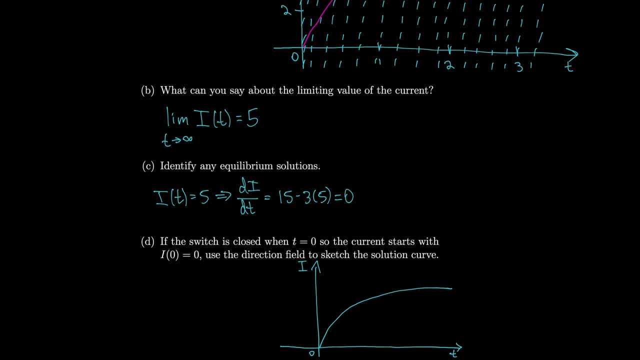 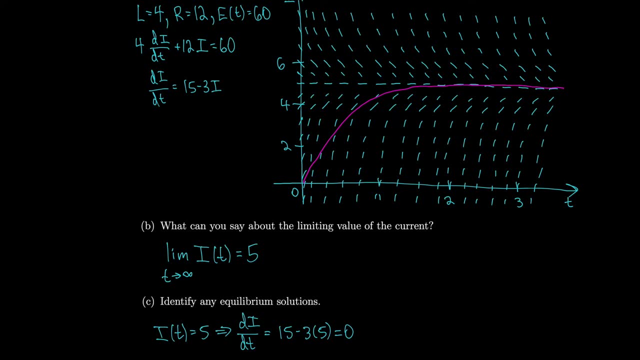 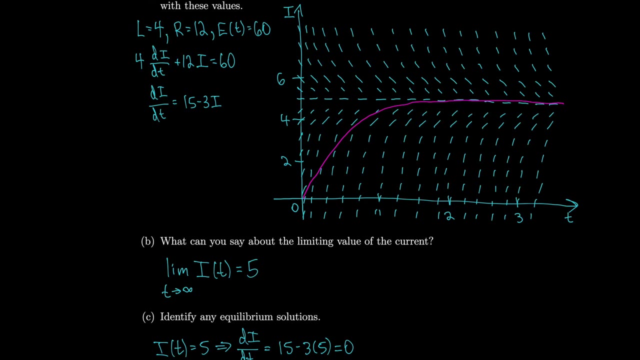 you could have tons of different solution curves, remember? it could have started anywhere, but we were just told: start at 0. in our case, this differential equation is called autonomous, because the independent variable is missing from this right side. as i said before, that's what made our equilibrium solution a nice flat line. 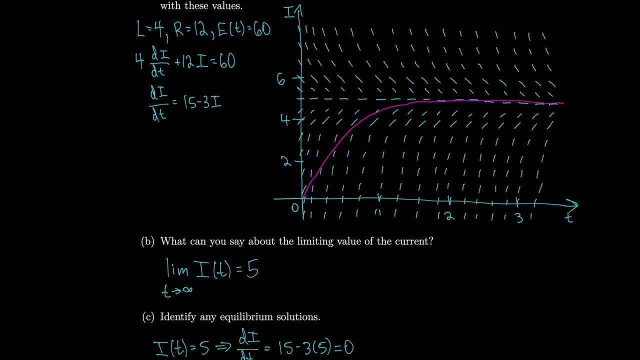 so when we have autonomous differential equations, that means that the slope at every single point corresponds to points with the exact same. well, i mean, when the y coordinate at every single point is equal, then the slopes of all those points correspond for all those little line segments. that's how we drew our slope field to begin with. 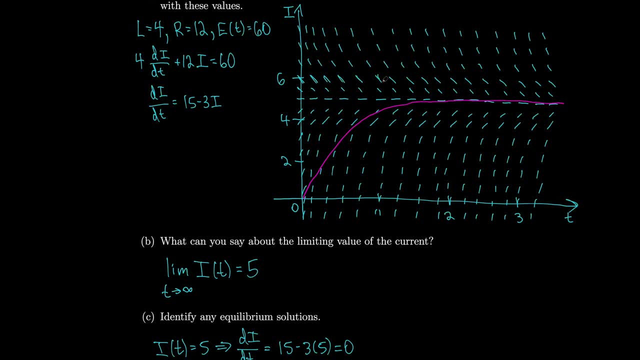 for every single one of these y values. all of our slopes are the same for any t value, which is what you have, which is what happens when you have an autonomous differential equation. so what this means is that if we have one solution to a differential equation, then we have infinite more solutions. 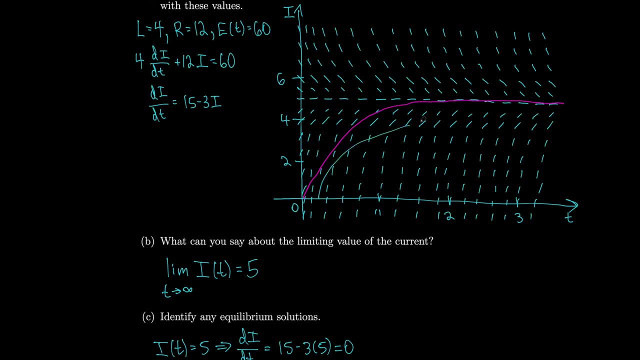 just by shifting our solution over. we can just maybe draw it a little better, so i could maybe shift over to 1, like that, and then i've got a solution by shifting my pink line over to 1, and then i could shift it over to 2. 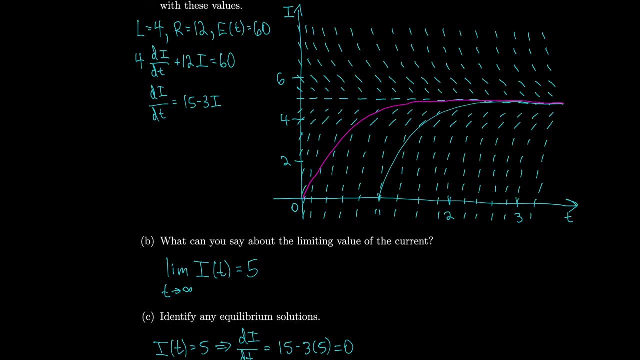 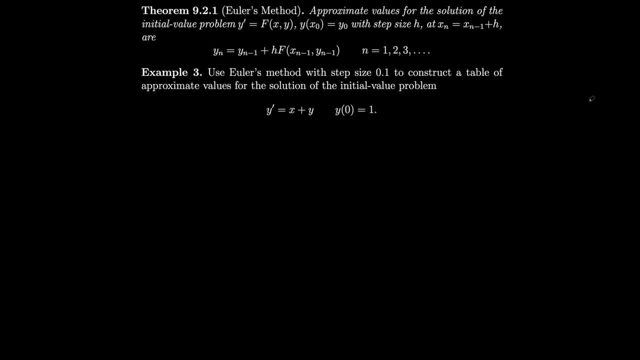 and i have another solution to my differential equation. Euler's method says that approximate values for the solution of the initial value y prime equals f of x, y where y of x naught equals y naught with step size h at x values x n equals our previous x value, x n minus 1 plus h. 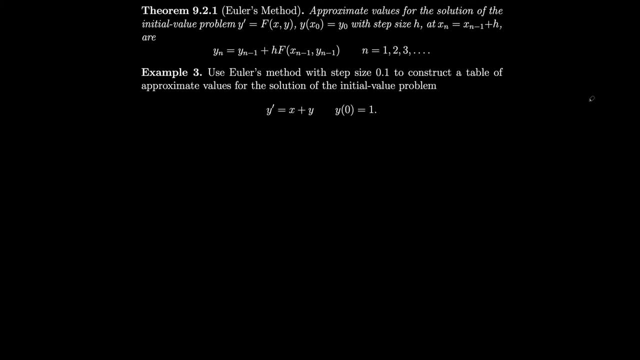 are y n, so our y value is equal to y n minus 1. our previous y value plus our step size. h times the value of the function at the previous y value. so this is very similar to Euler's method, as we did before, except that now. 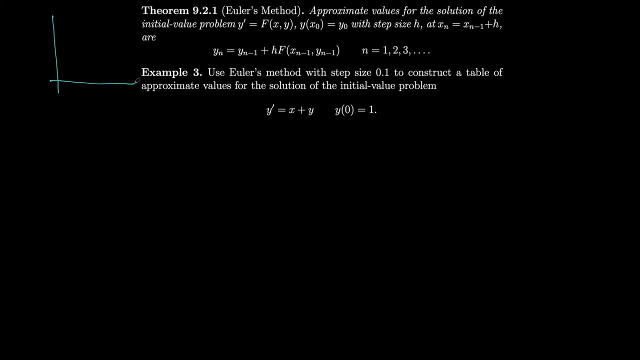 what we're doing is we look at the solution curve to a differential equation. so let's say: here's our solution curve, that's our. i can do it pink if you want it to be similar to what we did before. so we have a particular solution curve. 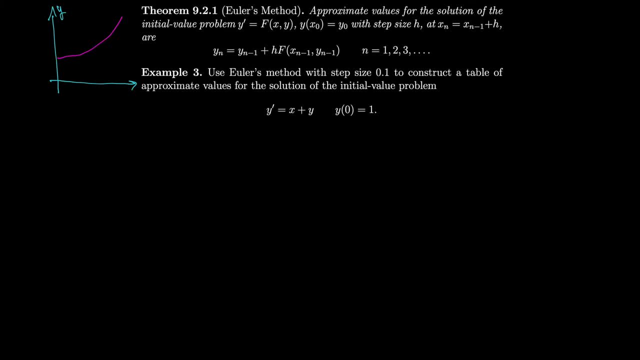 we want to try to approximate that solution. so what we do is we approximate it using linearizations. so we draw some line to approximate it, but then notice, if i keep drawing the line it becomes a very poor approximation the farther i go. so what we do is we stop. 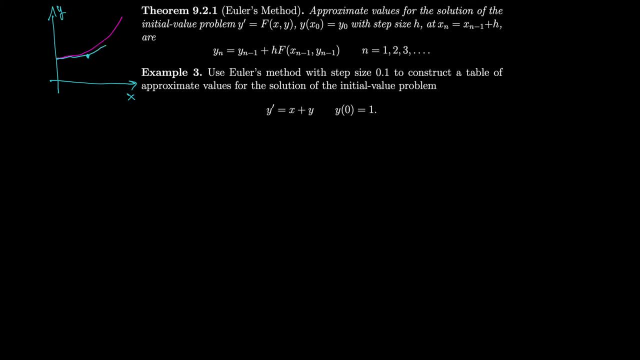 and we adjust and we draw another line, but then again we get the same issue. if i keep doing that it gets to be a bad approximation. so we adjust and we change it to another line, and we keep doing that, drawing more and more line segments for different linearizations. 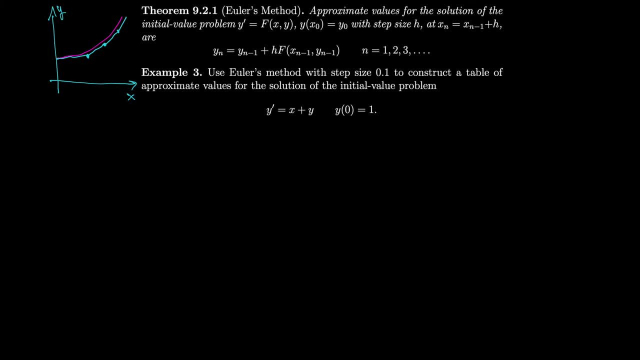 and we can keep approximating different y values this way for our solution. so we don't actually get an equation for the solution. what we do is we get a table of values that should hopefully match the table of values, or at least closely match the table of values. 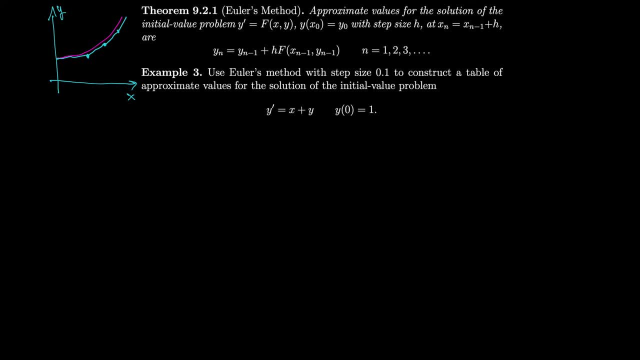 of the actual solution and if we want it to match closer and closer, obviously we make our step size h smaller, because the closer we get, the sooner that we pivot and draw another line segment. the more line segments we draw, the better our approximation becomes. notice that this looks a little bit scary. 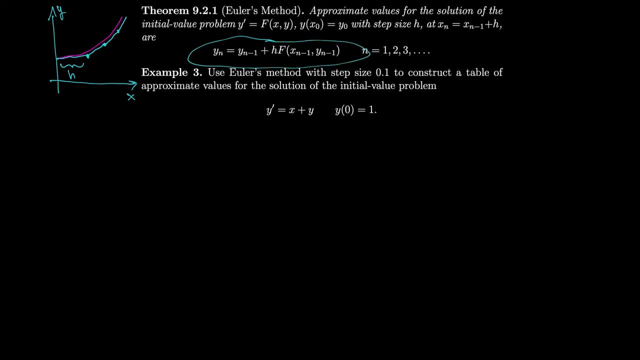 and looks a little bit like a mess, but it really is just a linearization. remember that for point slope form we have: y minus y1 equals our slope m times x minus x1, which was our linearization essentially. also remember that our slope is our derivative. 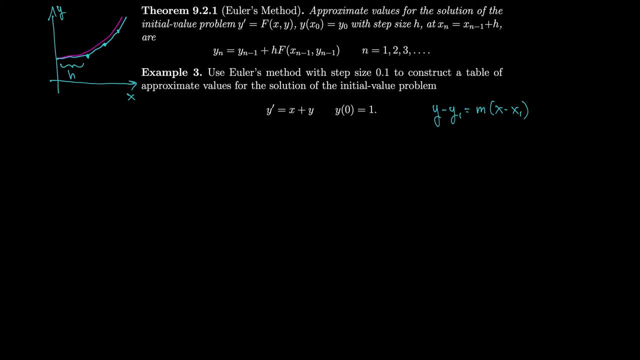 f is our derivative. that's what differential equations are. so that's where this m comes in. that's f. our change in x is our step size, h, and our y1 is just on the other side. you can just move it over, so let's use this linearization. 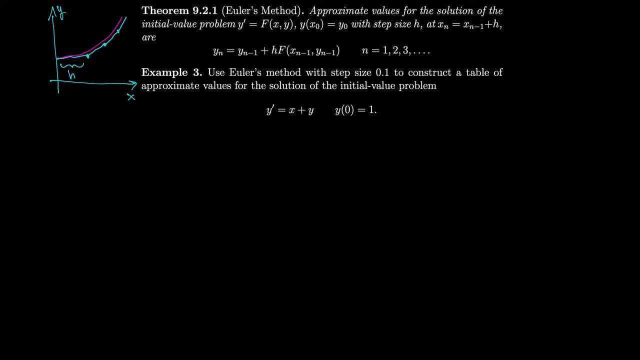 to come up with a table of values to approximate the solution for the initial value problem. y prime equals x plus y, where our initial value y is equal to 1. so how about we do a step size of 0.1? that should be pretty accurate. 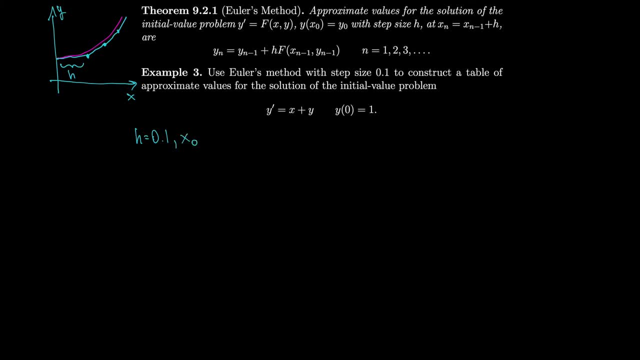 accurate enough, and our starting x value is 0 and our starting y value is 1, then our function or our derivative, which is slope of the tangent line, is x plus y. so let's get. well, we started with one point over here. we know that 0 comma 1. 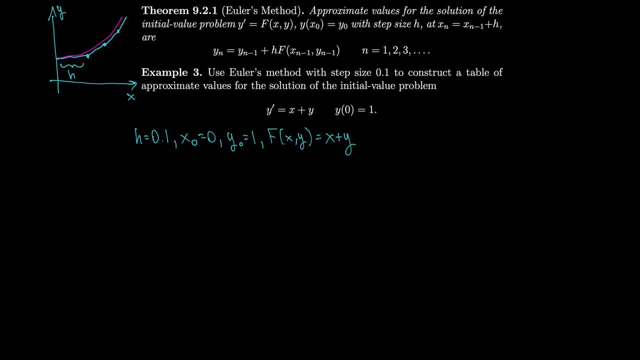 is definitely on our solution. so let's get our next point. so we'll get y1. now. that's equal to the previous y value plus our step size: h times f of our previous point, x naught, y naught. so our first y value is 1. 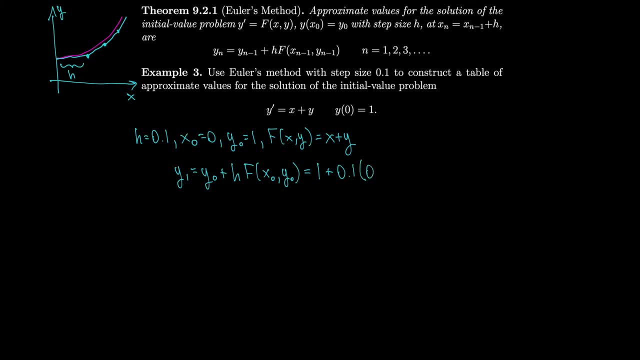 our step size is 0.1. first x value is 0 and y value is 1, so we get 1.1 for our y1, our second y value. let's get y2 now, so y2 will be y1, our previous y value. 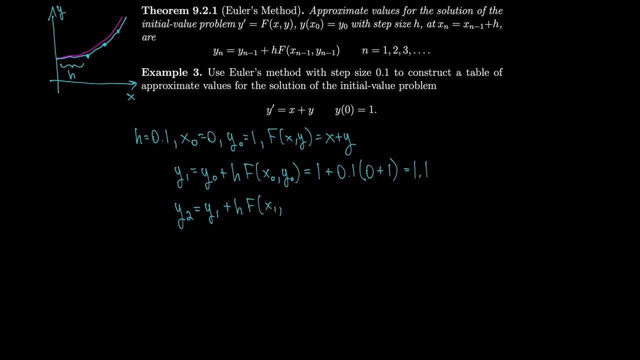 plus our step size times f of our previous point, x1, y1. so now notice we're plugging in y1, so we plug in what we just solved for, which was 1.1, and we use our step size of 0.1 again. 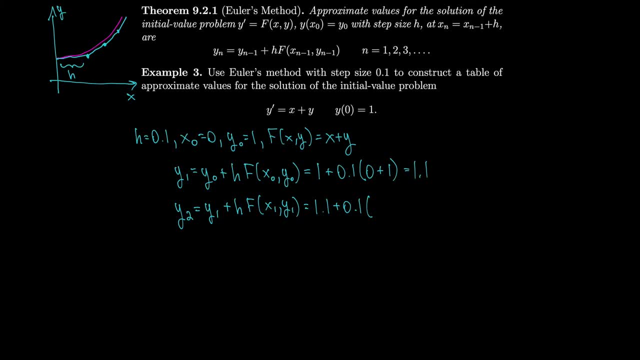 but notice now: we need x1, y1 in the start of our function where we add them together. so if our first point was at 0, so that would be 0 over here and then we move over h. that means that our second x value is 0.1 more than 0. 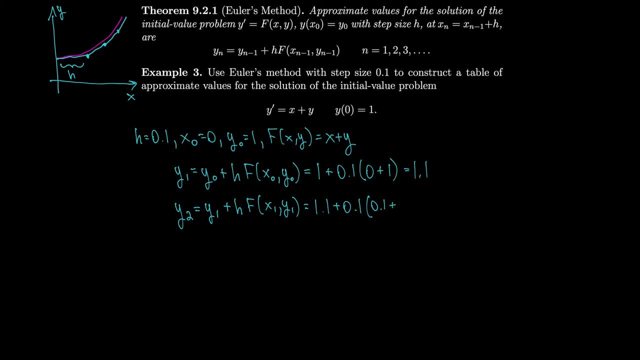 so our second x value is just 0.1 and we already know our second y value is 1.1. so that ends up being 1.22 for y2. for y3 we do the same process again: y2 plus h times f of our previous point. 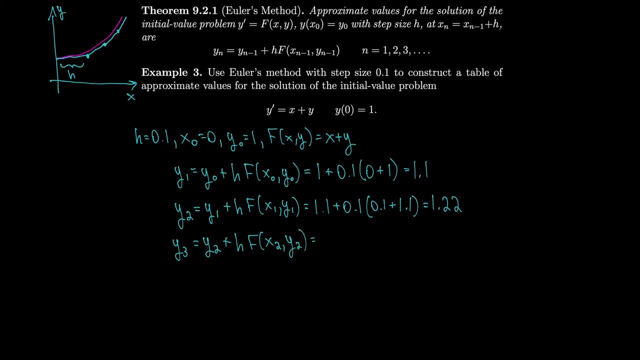 x2- y2, we get 1.22, because that's where y2 was, plus our step size, 0.1 times our next x value. if the first x value is 0, then it moved up by 0.1. the next one will move up another 0.1. 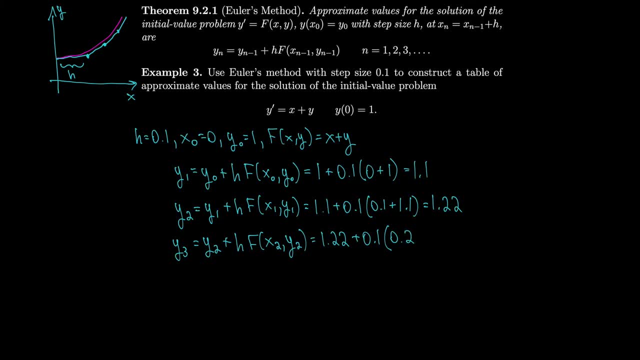 because that's what h is doing, and our next value for x would be 0.2. we add that to our y value, because that's what our differential equation is telling us to do, and we get 1.362 for y3. so what this is saying is that 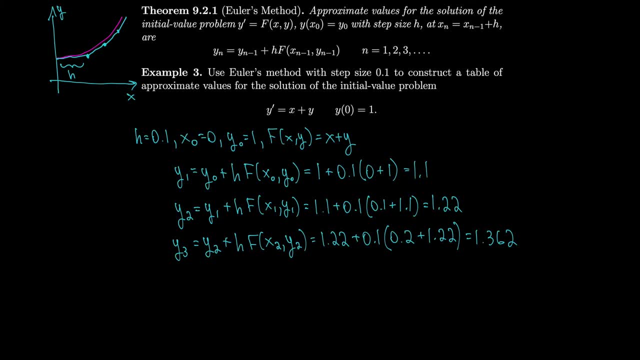 for our solution curve y is absolutely equal to 1, y of the next point, y of 0.1 is approximately equal to 1.1 on our purple line using the blue one, then y of our next x value, so y of 0.2. 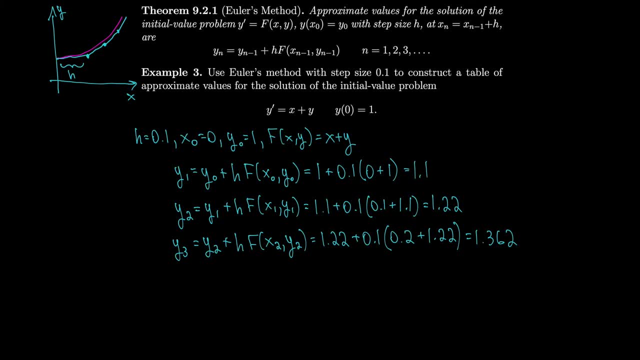 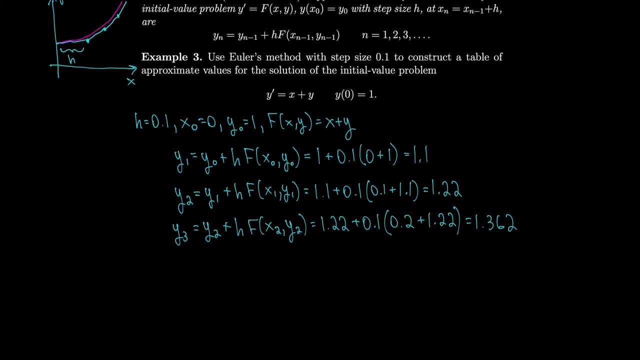 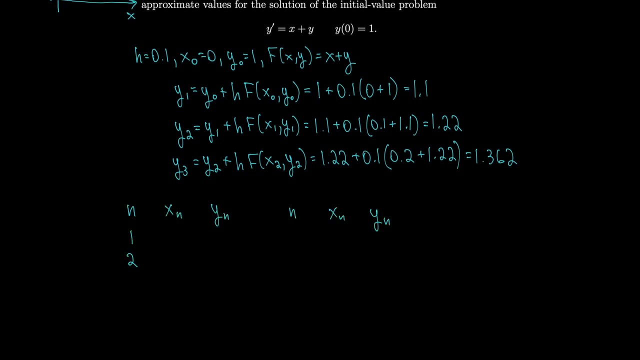 is approximately 1.22, y of 0.3 is approximately 1.362. so if we do that, if we keep doing this process over and over, we can get a nice table of values. so how about I draw that? so you should end up with a table of values. 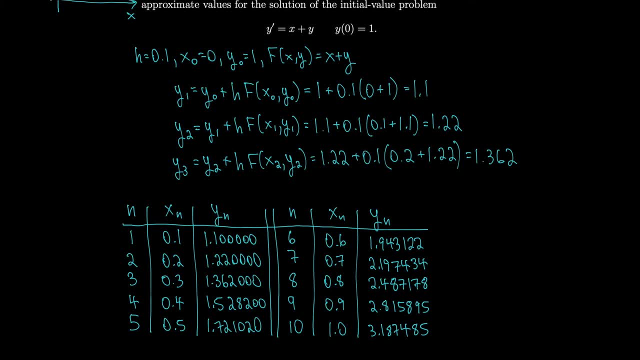 that looks something like that and remember what this means. this means that these values approximate the table of values we would get if we were actually looking at the solution curve itself, instead of just approximating it. so we would expect that on the solution curve, for example, the actual y value, 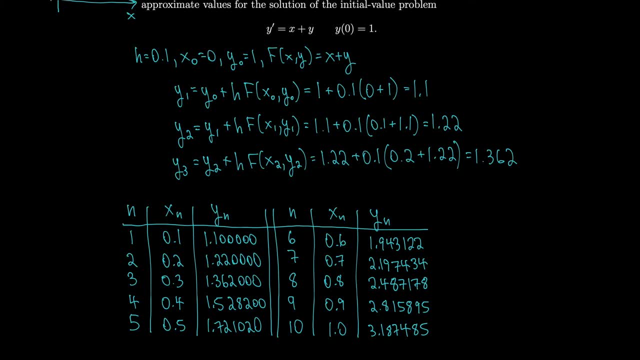 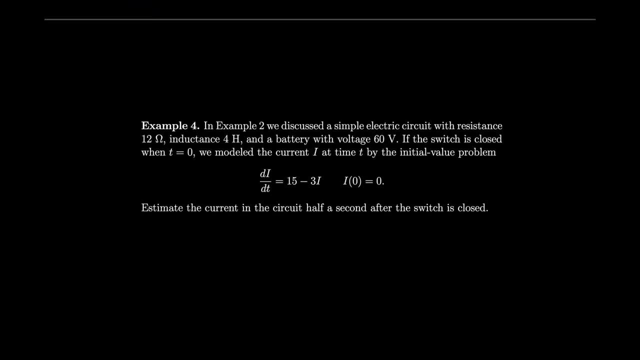 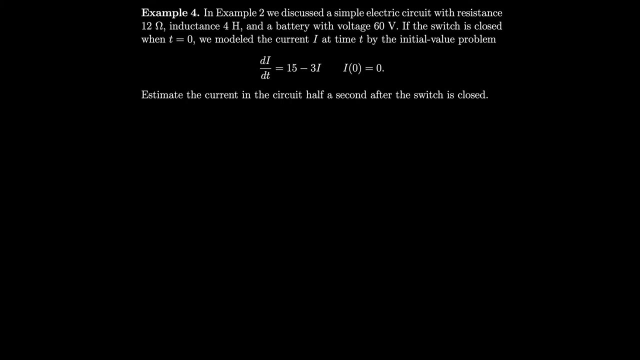 at 0.8 would be approximately 2.487178. in example 2 we discussed a simple electric circuit with resistance 12 ohms, inductance 4 henries and a battery with voltage 60 volts. if the switch is closed when t equals 0. 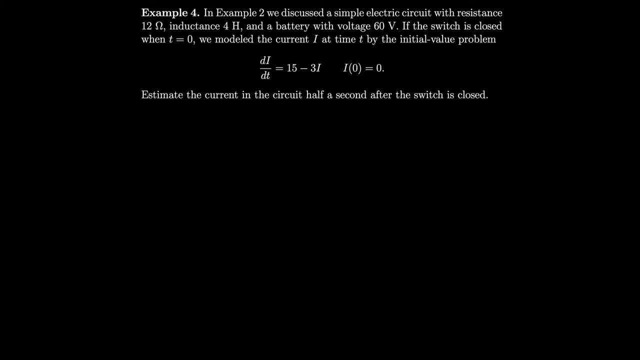 we model the current i at time t by the initial value problem d i, d. t equals 15 minus 3 i where i of 0 equals 0. let's estimate the current in the circuit half a second after the switch is closed. so we're estimating values in our solution curve. 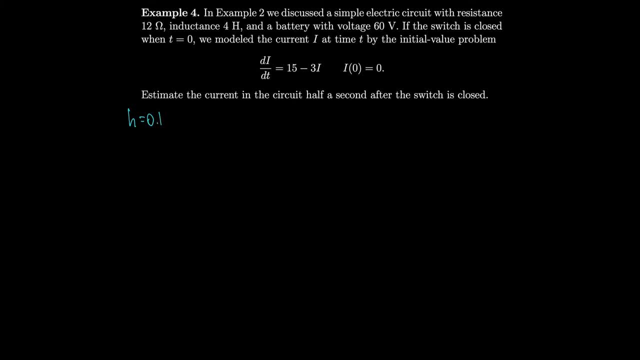 that we drew in purple, so pink or whatever color it is, I don't even know. so h will choose to be 0.1 again for our step size. we'll start at time 0 and we'll start at i of 0, which is 0. 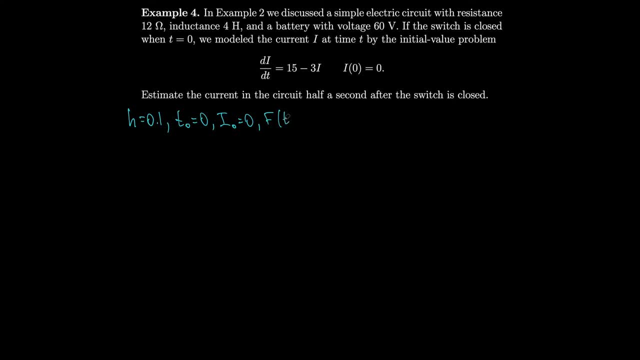 and we will look at f of t, i, which is our differential equation, or the right side of our differential equation. so let's use Euler's method. let's look at our next. i value i of 1. that's going to be our previous one- 0. 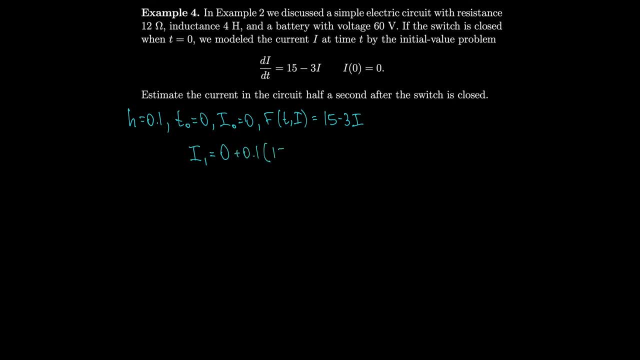 plus our step size, 0.1 times 15, minus 3 times our i value of 0, because that's what our previous i value was. so that's 1.5, and next for i of 2: we get that it's our previous one, 1.5. 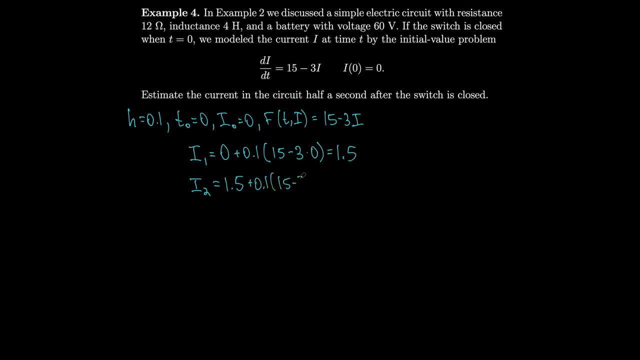 plus our step size 0.1 times 15, minus 3 times 1.5, which is 2.55. and we keep doing this, we get i of 3, which is 2.55 plus 0.1 times 15.5. 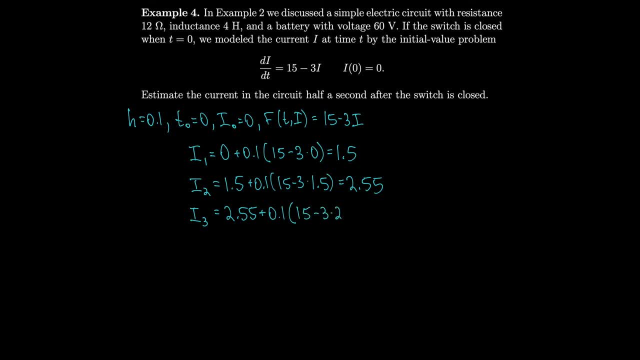 minus 3 times 2.55, so 3.285 i of 4 is 3.285 plus 0.1 times 15, minus 3 times 3, i think it's 3, it's 3.285. yeah, i was about to plug in 2.55 again. 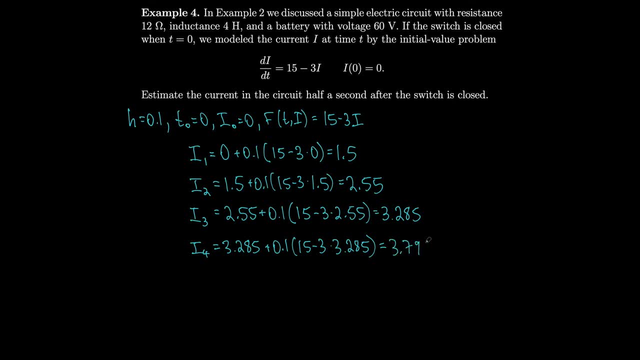 and we get 3.7995, and then i of 5 can be our last one, because it said we only needed to go half a second. so we were doing a step size of 0.1, which is a tenth of a second, so 0.5 will be. 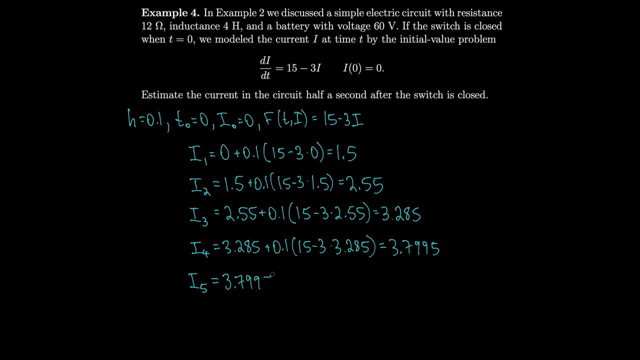 all we need, thank goodness. i don't know which is worse, this or the drawing. actually, no, the drawing is definitely worse. so 15 minus 3 times 3.7- 9.95, we get an approximation of 4.15- 9.65. 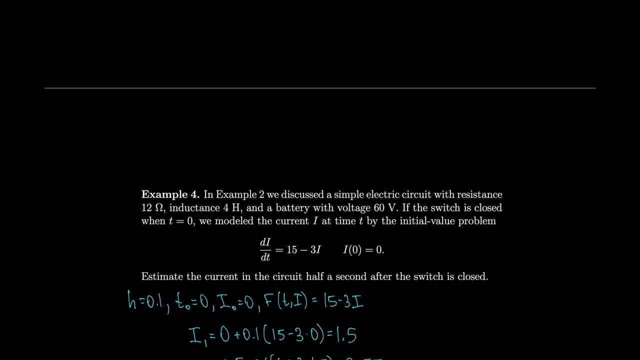 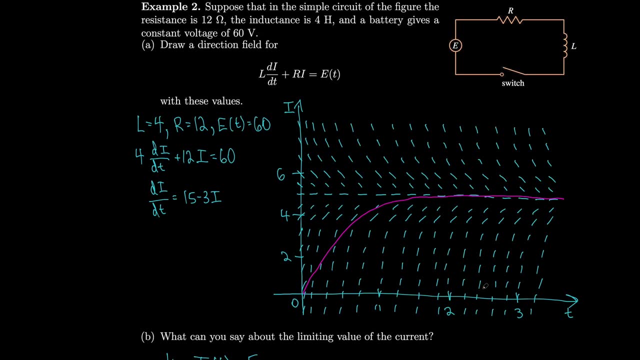 after half a second. let's go and take a look and make sure that that makes sense. take a look at our solution curve. so we were trying to approximate half a second, so that's roughly over here if we go up. i didn't draw it perfectly so it looks like it's around 4. 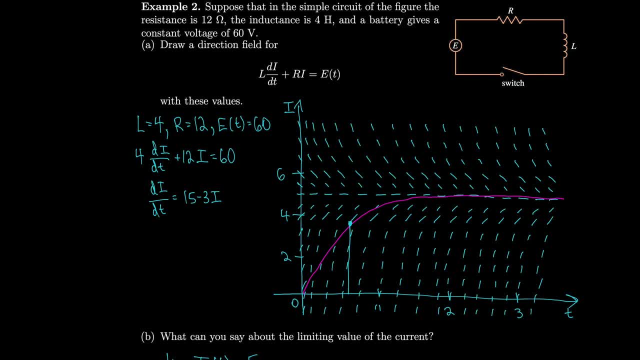 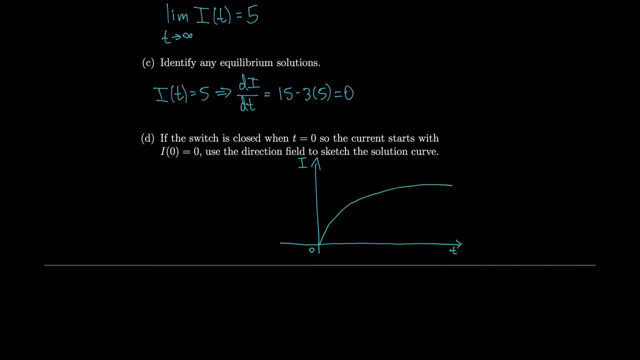 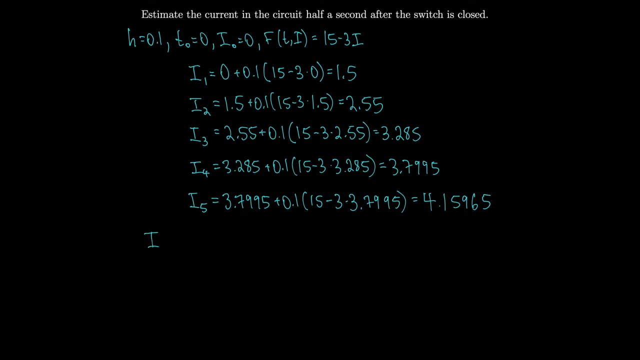 maybe i got skewed a little bit. probably should have drawn this going up a little bit higher, but yeah, it's about 4.16. we could say so in conclusion. how about we write that i of 0.5 is approximately 4.16 amps?